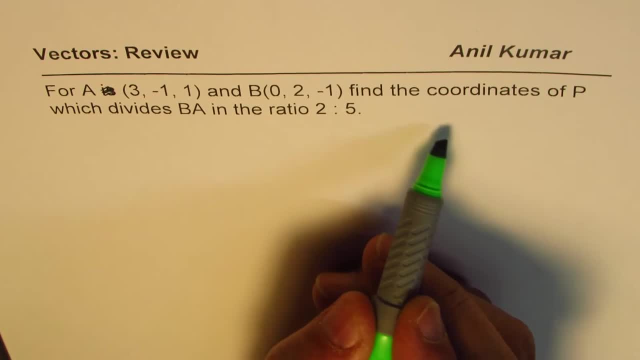 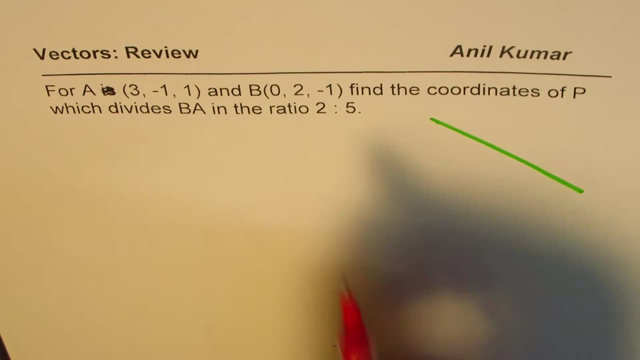 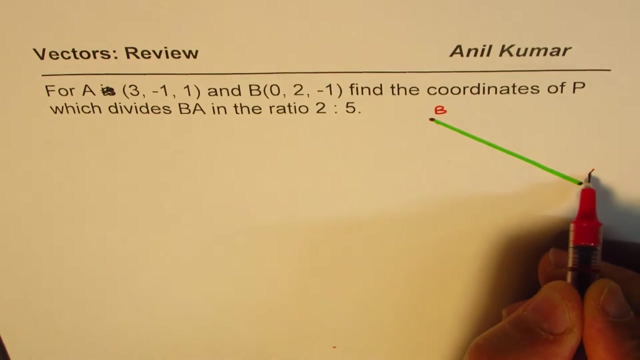 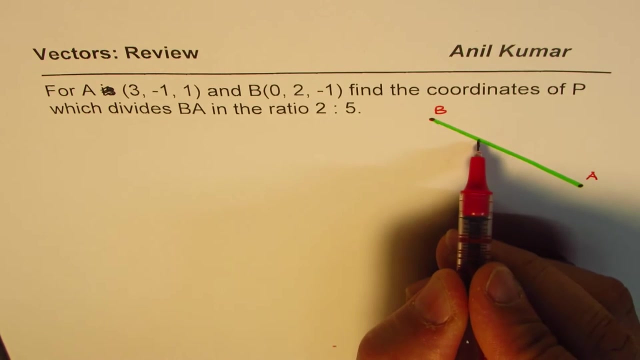 Let me sketch, describe the scenario first, right? So let's say that's the line we're just sketching at random and we want to divide line BA. So let me consider this point to be B and this point to be A. We need to divide it in the ratio of 2 is to 5 and some point P. let us say point P is right there, which divides BA in the ratio of 2 is to 5.. 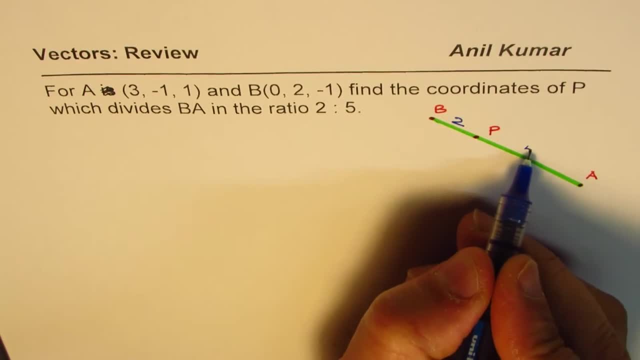 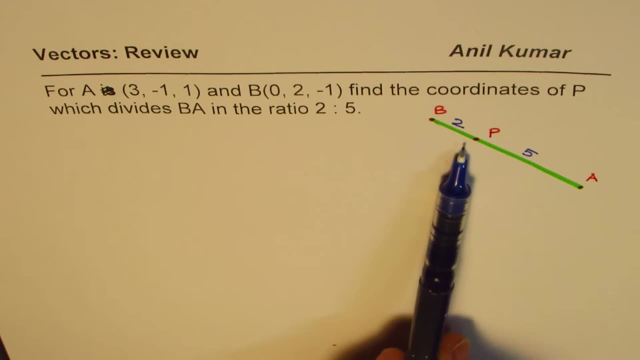 That is to say, that is how it is being divided, right? So the line segment BA is divided into 7 portions. BP is 2 out of those 7 and PA is 5 out of those. Okay, Now we need to find the location of point P, the coordinates of point P. That's the question for you, So you can actually pause the video, answer the question and then look into my suggestions. 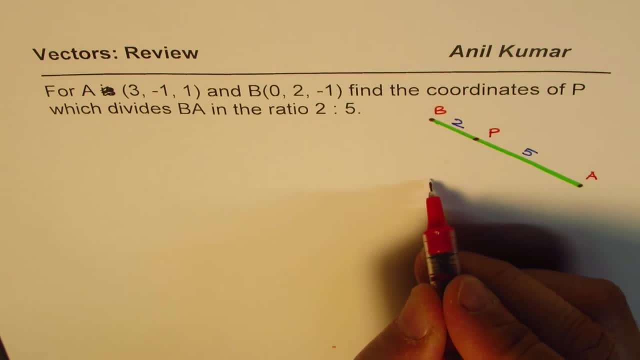 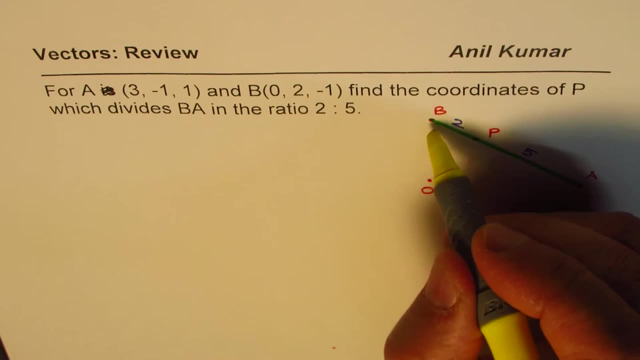 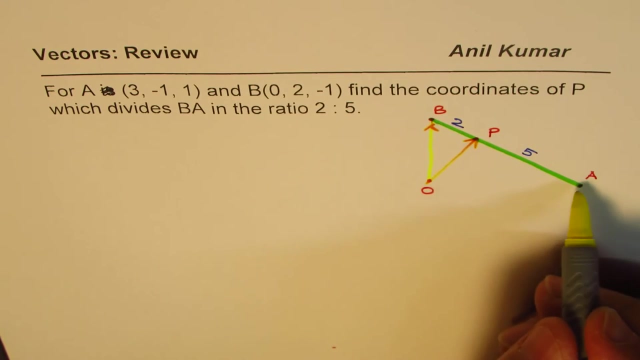 Now let us assume that we have somewhere here origin. Let's say this is the origin for us. In that case, the vectors we are considering is the position vector OB, that's the position vector, And we have position vector OP And we also have the position vector OA, right? So these are the position vectors which we are going to consider. 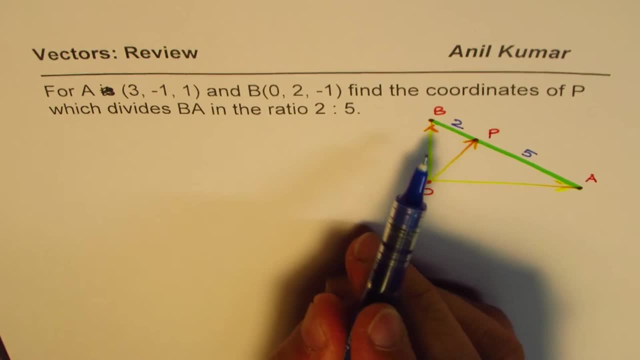 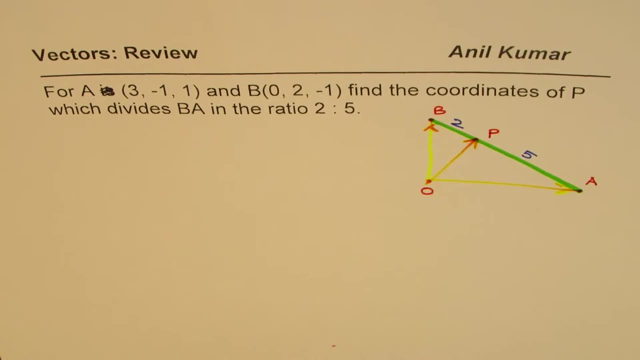 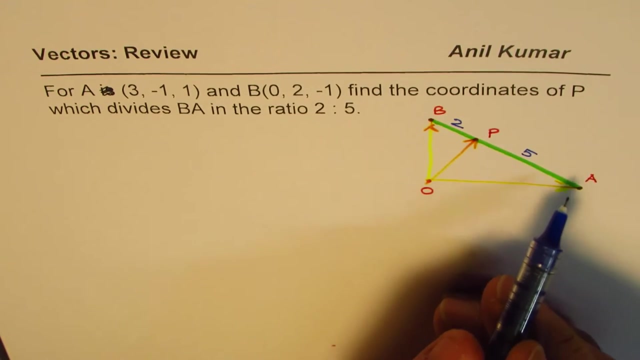 Now let us say that we will derive the formula first. I could use the formula and find the answer immediately, no problems. But what I will do here is that we'll kind of derive the formula right. So what we can do is let us say: let's take the formula in general, That is to say that if we have 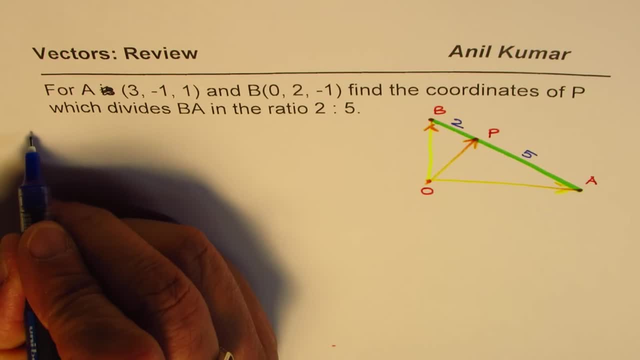 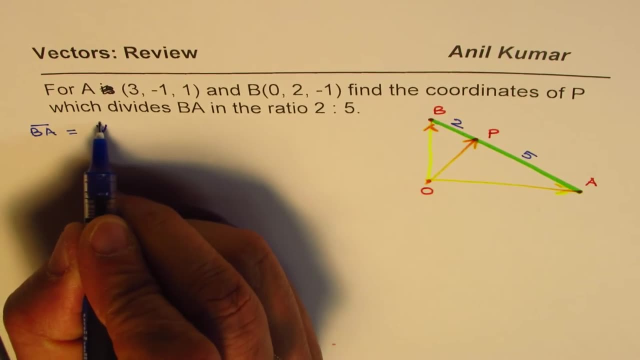 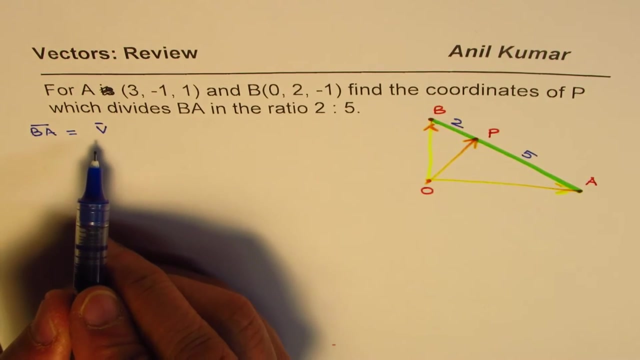 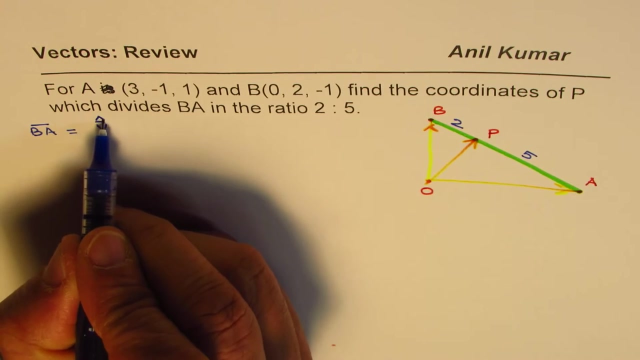 BA. we could denote BA as, let's say: in general: we'll say: BA is some unit vector V, right, Let's say V is the unit vector in the direction of BA. I'm first trying to give you a proof. okay, In that case we'll say: unit vector along BA. we can denote by this: that is the unit vector along BA. let us say: 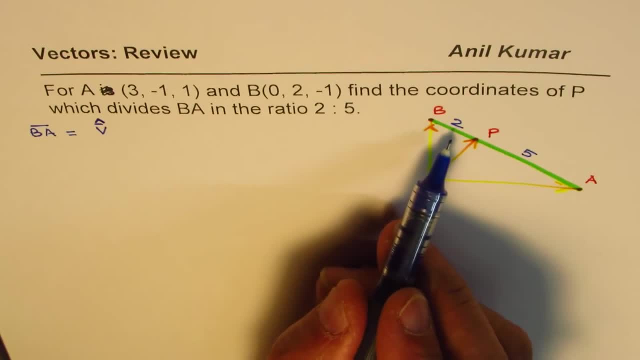 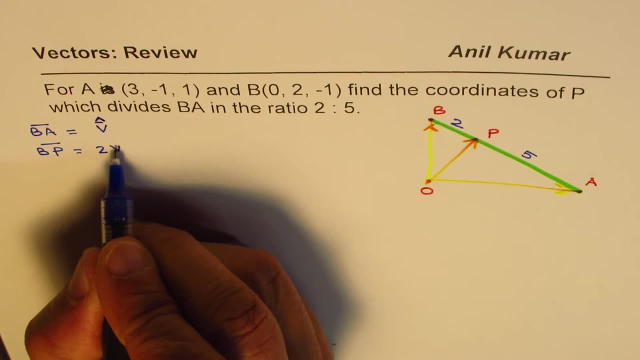 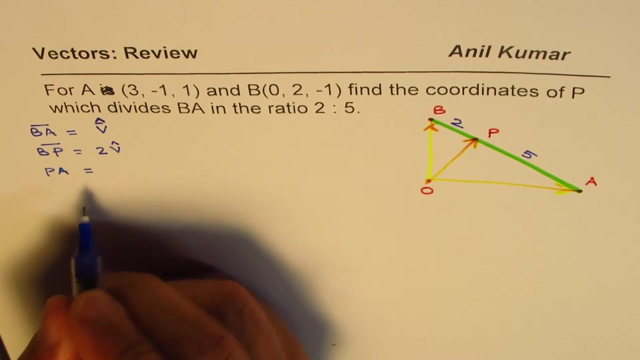 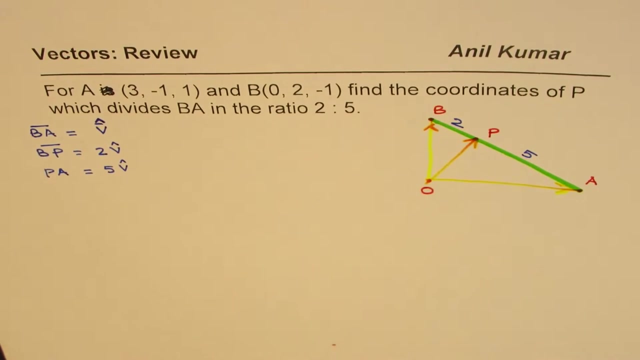 Okay, In that case, what we have is that B- P could be written as 2 times this unit vector, correct, And P- A will be equals to 5 times this unit vector, correct. So that is how this unit vector will be. 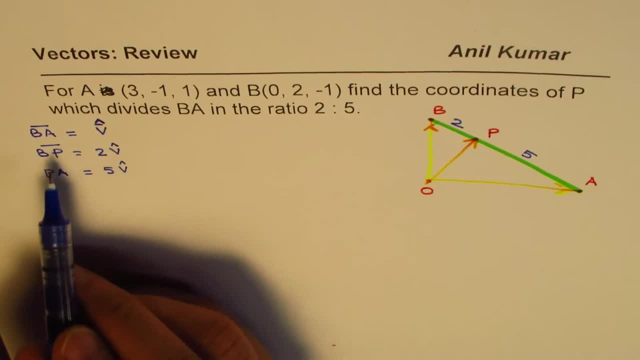 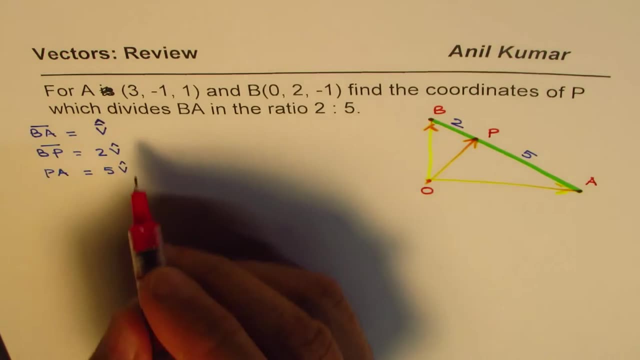 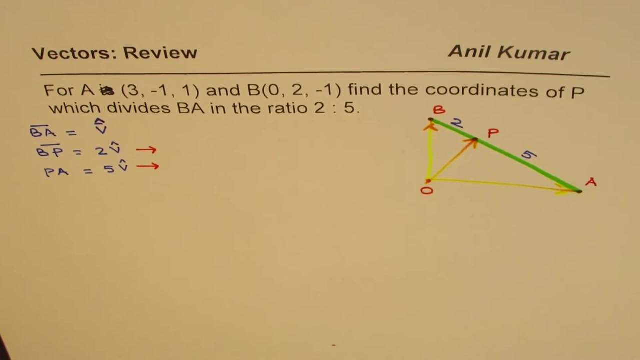 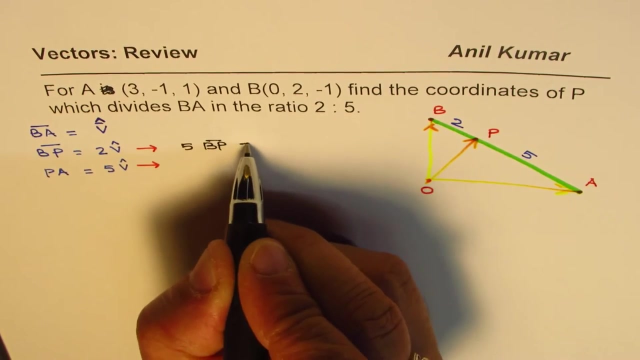 Now, if I multiply the first equation by 5 and the second by 2, what happens, See from here. if I times the first equation by 5, let me write in a different thing: 5 times, I get. 5 times B. P is equals to 5 times 2, is 10, V, right, And then I get the second equation by 2, what happens? See from here, if I write in a different thing 5 times, I get 5 times B. P is equals to 5 times 2, is 10, V, right, And 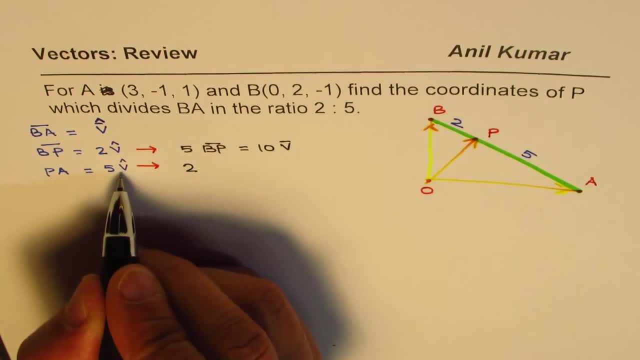 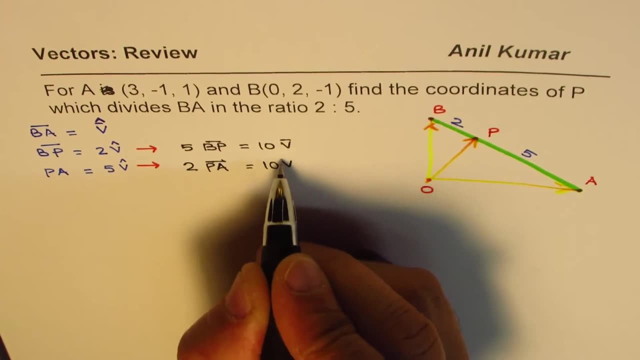 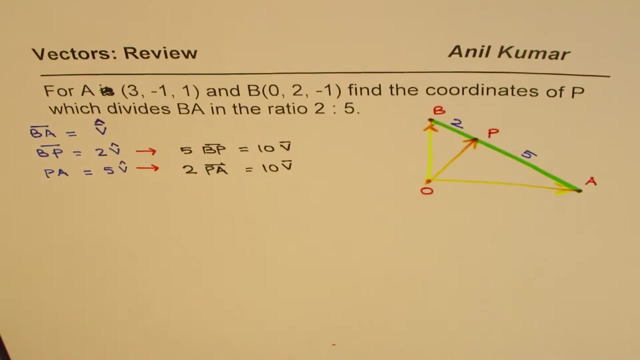 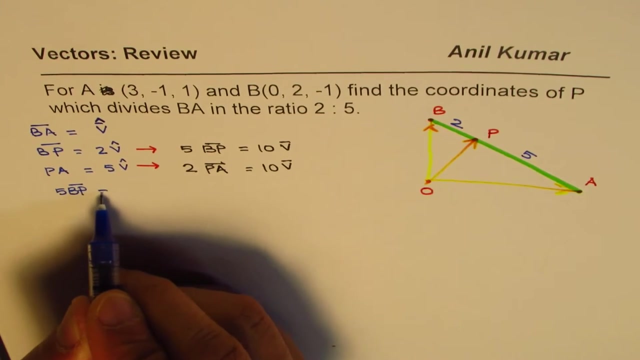 And the second one I get 2 times. if I multiply this one by 2 times P A, we get 10 V right. So that indicates that these 2 parameters are equal right. So from here we can clearly write that 5 times B P is equals to 2 times P A right. 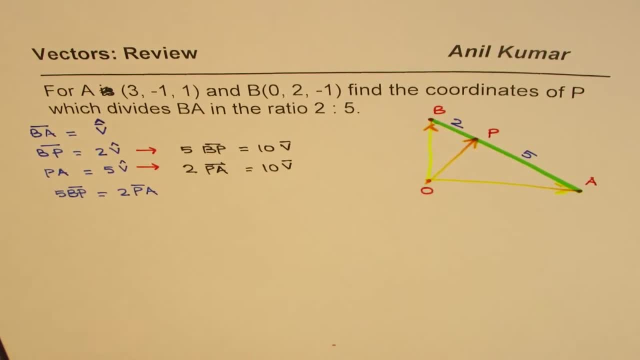 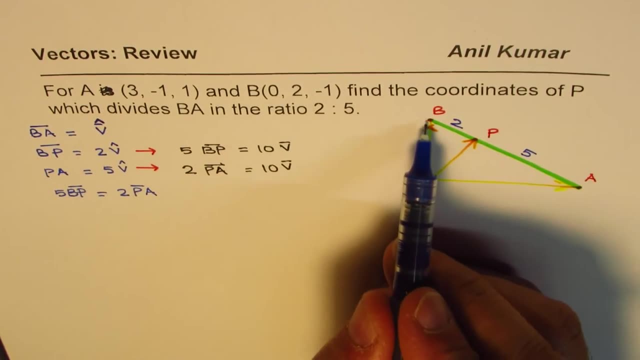 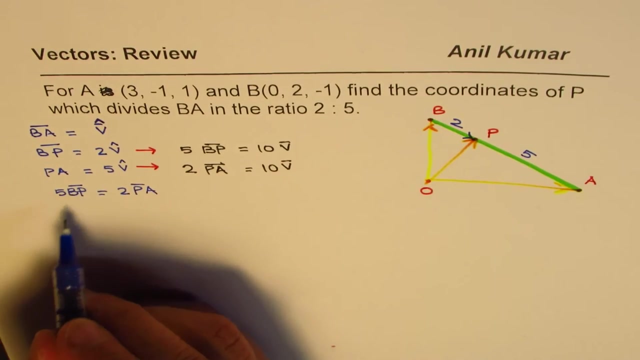 So you see how this unit vector helped us to form an equations very critical. ok, Now what is B P, B to P? we are talking about this now. B P is O P minus O B. right, So I can replace B P by 5 times O P minus O B. 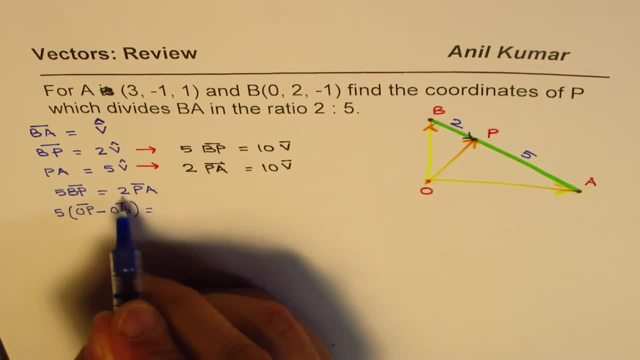 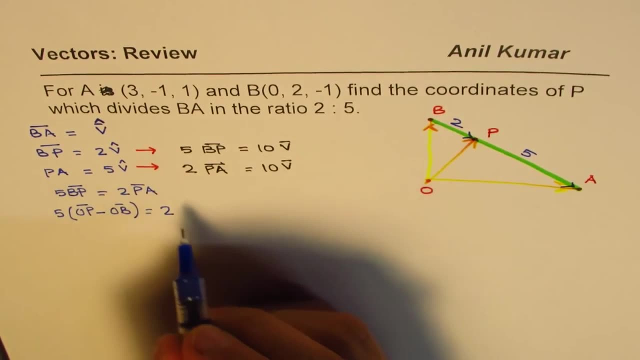 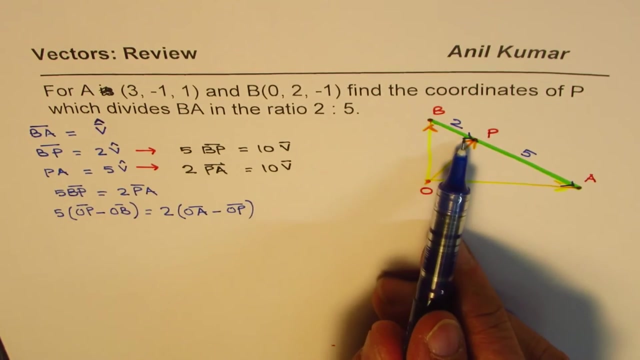 So we have related this in terms of position vectors. Do you see that Right P A, so P to A, is O A minus O P, right? So 2 times O A minus O P. do you get it? So what we did was first we proved that 5 B P is 2 P A, and then we wrote B P, B to P. 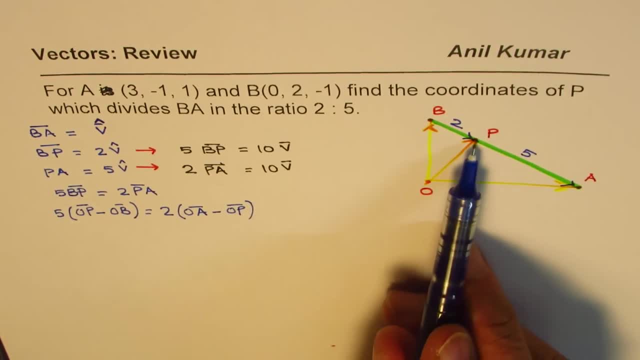 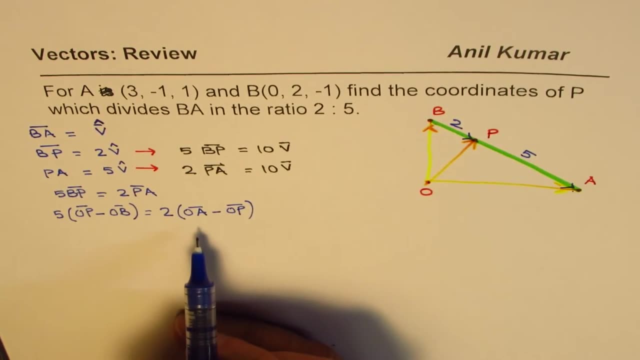 as O P minus O B, and P to A as O A minus O P, correct? So we got position vectors. now What do we need to find? We need to find coordinates of P, right, that is what we need to find. So from here we can isolate P. So let me open the brackets 5 times O P minus 5 times O B. 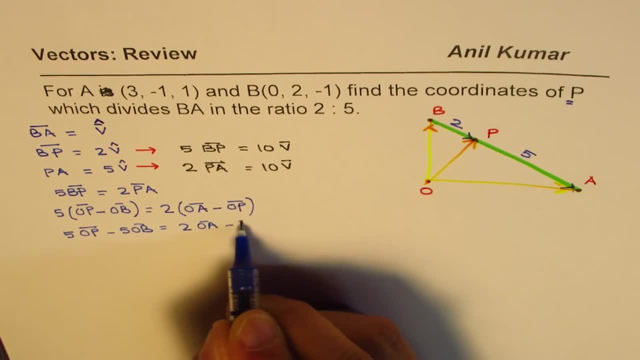 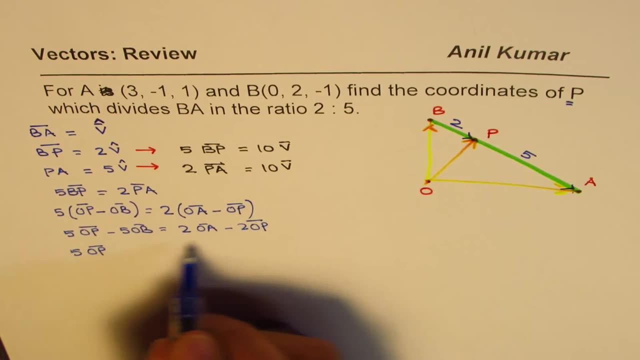 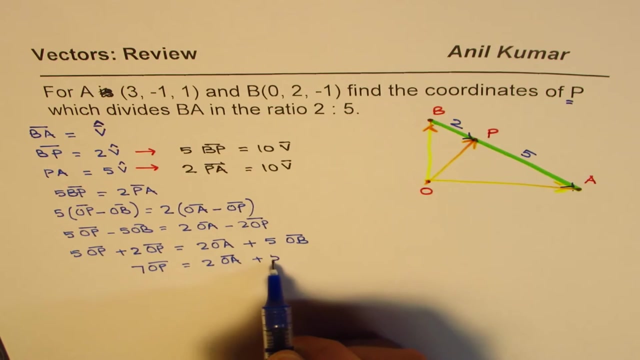 equals to 2 times O A minus 2 times O P. Bringing it to the right side, 5 times O P plus 2 times O P is equals to 2 times O A plus 5 times O B. right Now that is 7 O P, right? 7 times O P equals to 2 times O A plus 5 times O B. perfect. 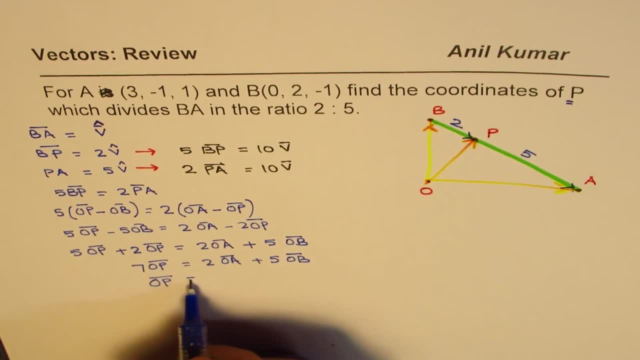 Now what is O P? So the position vector O- P is dividing both by 7.. So we get 2 over 7 times O A plus 5 times O B. right Now, what is O P? So the position vector O- P is dividing both by 7.. 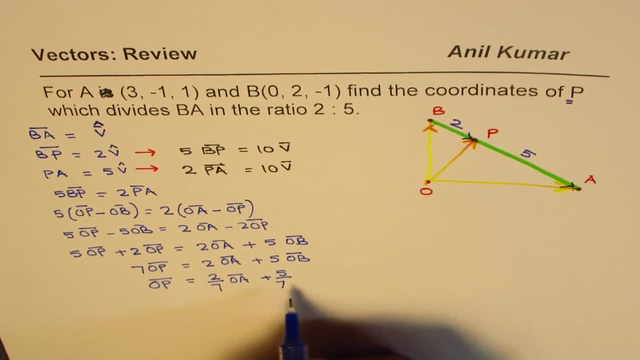 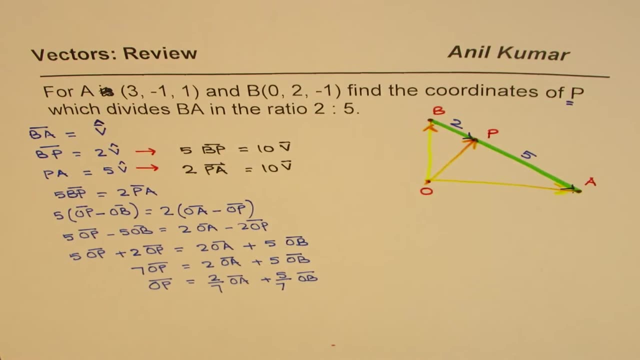 So we get 2 over 7 times O A plus 5 times O B plus 5 over 7 times O B, right? So that is how we get this particular relation. So position vector P now can be found easily where, in our case, we have taken the ratio. 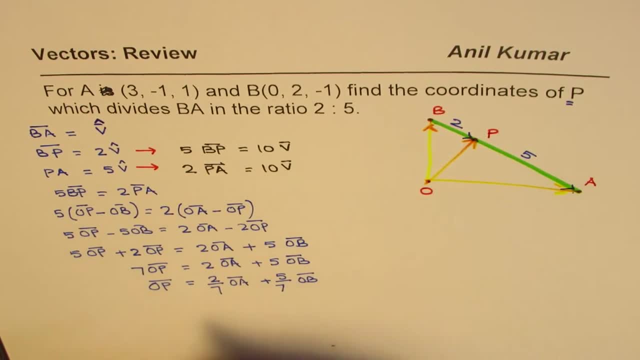 2 is to 5, but in general, if we have a ratio of M is to N in general. in that case this formula: See O- A when I am multiplying with, See O A. when I am multiplying with, I am multiplying by 2, right. 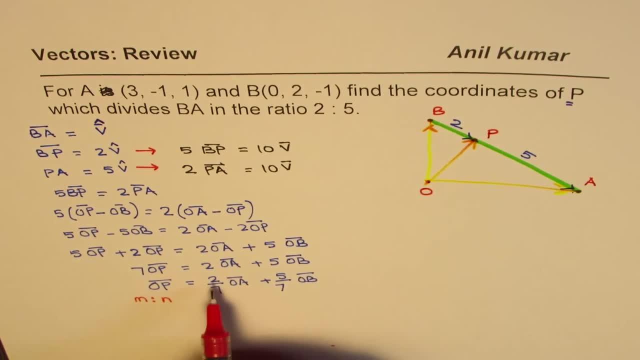 So in that case, if I do, instead of 2, O is to 5, if I do M is to N, then general formula will be O- P for the given diagram. if I make this as M is to N, ok, Then you know this is M right. so M over 7 is combination of these two right. 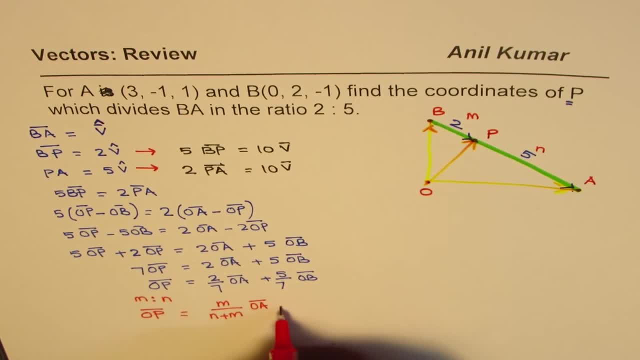 So N plus M times O A, N plus M times O A. So this is M right plus n over, n plus m times OB. so that becomes a general formula which can always be applied for such situations, right? so? so whenever we are dividing a 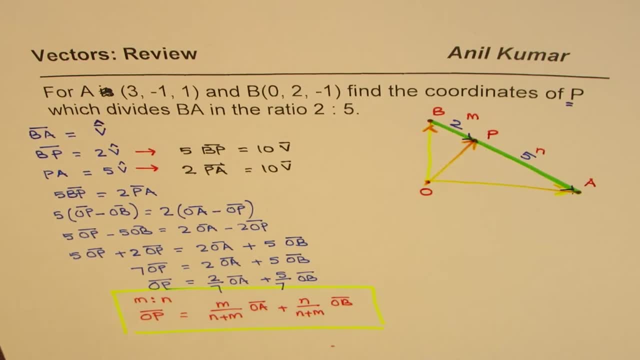 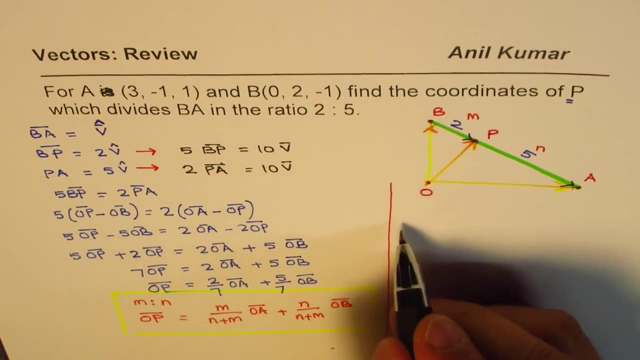 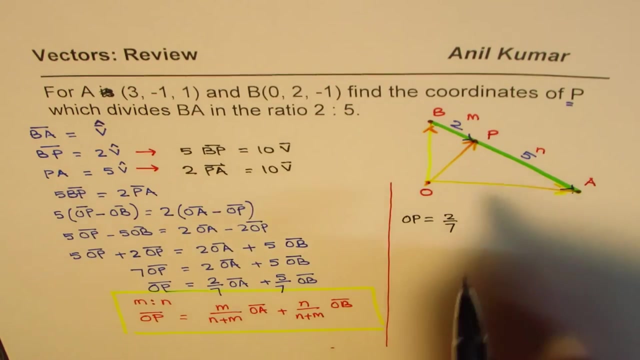 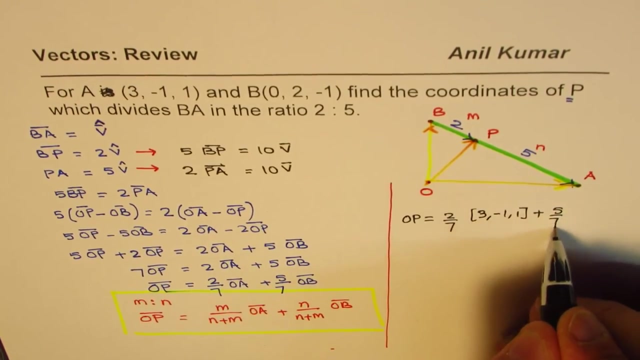 line segment in a ratio. we could apply this form. okay, now let us apply the formula and get the result. so OP is equals to 2 over 7, and what is OA? OA is 3 minus 1- 1, so we can write this as 3 minus 1, 1 plus 5 over 7, and OB is 0- 2. 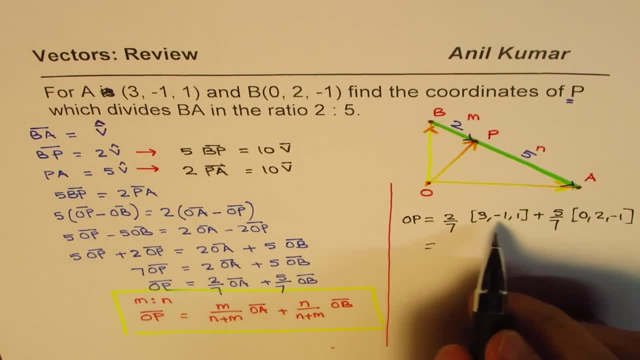 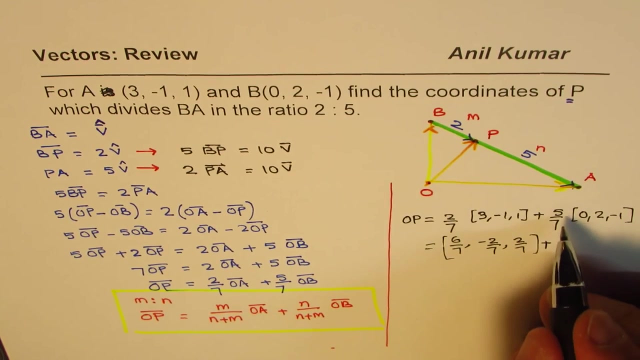 minus 1. okay, now you can multiply all these numbers, so we get 2 times 3 is 6 over 7, 1 1 2, 7, 1 minus 2 over 7, then again we have 2 over 7, so that is plus, that is 0, and this is. 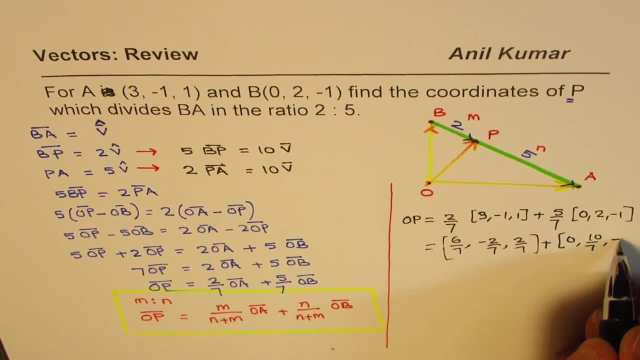 10 over 7, minus 5 over 7, correct. Now we can combine them. so 6 plus 0 is 6, 6 over 7, minus 2 plus 10 gives us 8 over 7, and 2 minus 5 gives us minus 3 over 7.. So that: 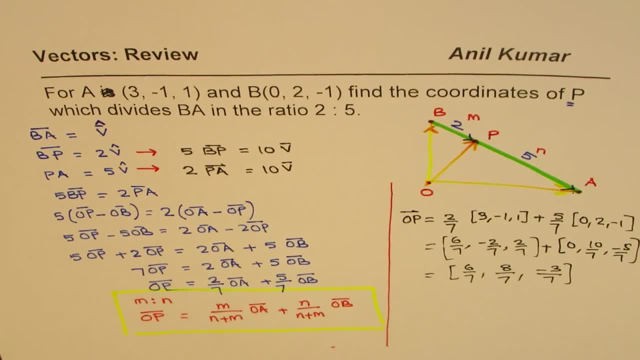 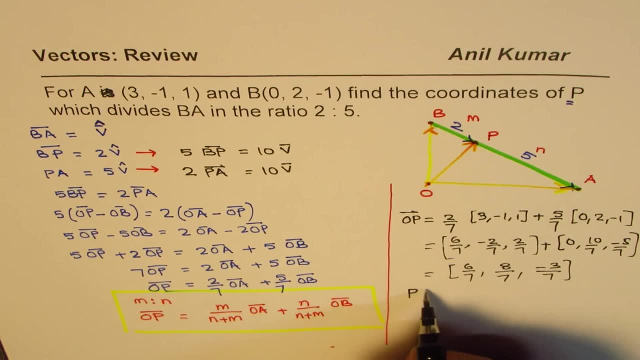 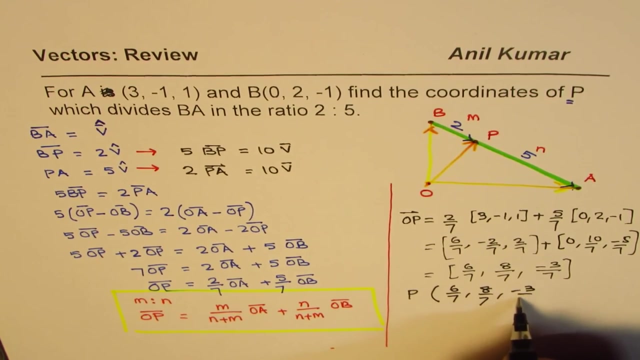 becomes the position vector of P. So now we know the position vector, we need to write coordinates, important, right. So the coordinates P will be 6 over 7,, 8 over 7, minus 3 over 7, right. 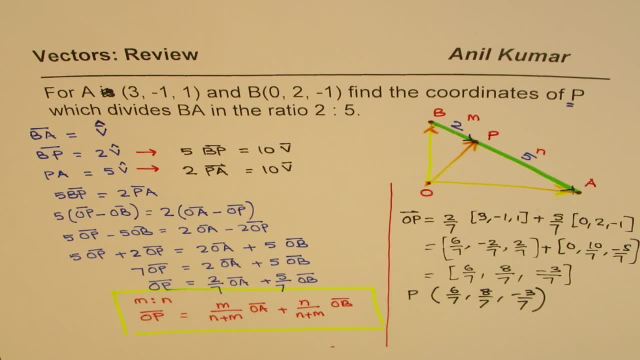 So that is how you get your answer. I hope the steps are clear and you could do any question related with division of line. I'll provide you a link with external division also. this is we call it internal, So P is in between B and A, right, So internally it. 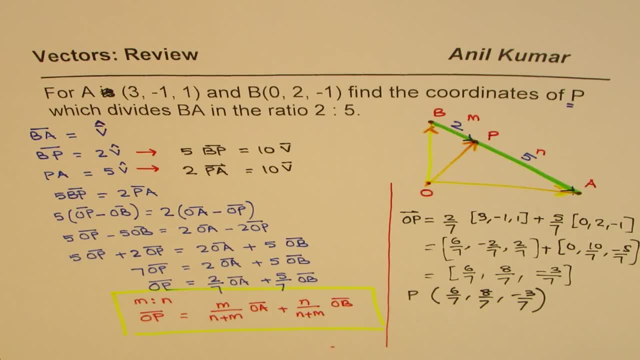 divides into the ratio of M is to N. Now in your test you could get P dividing externally. Well, the formula remains the same. you could always use the same formula, but you could use this formula to get the result. I'm Anil Kumar and I hope that really helps You can.